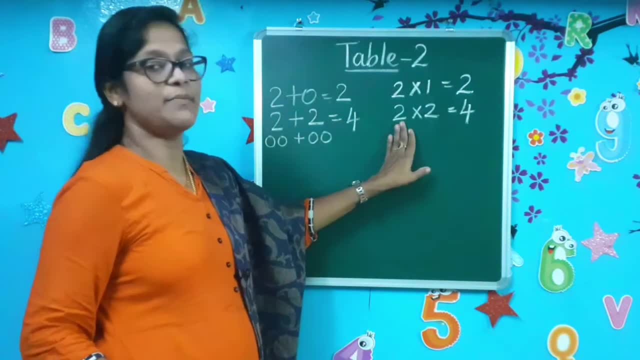 plus 2, it's 4.. And when you multiply, it's 4.. So when you add 2 plus 2, it's 4.. So when you multiply, 2 is the table, 2, table into 2.. 2, 2s are and in twice. when you multiply it, it's 4.. 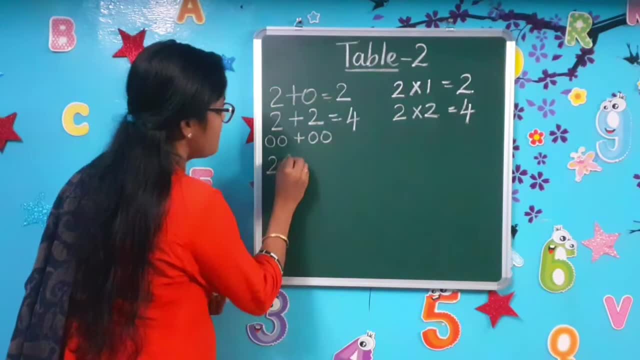 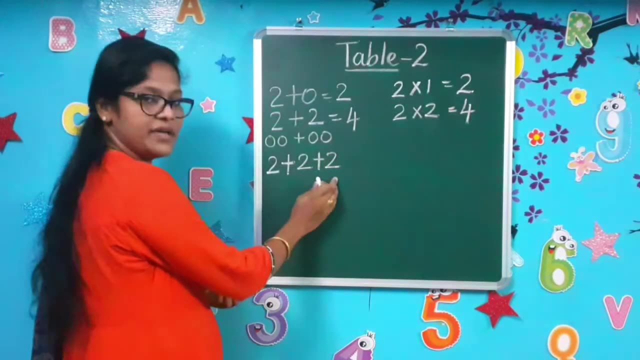 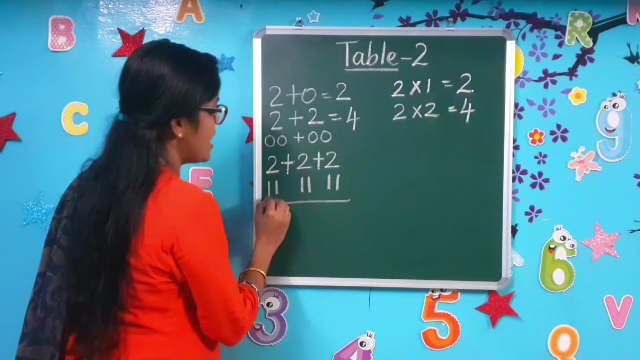 Okay, come on, let's see it again: 2 plus 2 plus 2.. So, thrice, 1, 2, 3, 2s are here, So you have to add them. Okay, come on, let's draw the lines and count them. Okay, 1,, 2,, 3, 4, 5, 6.. So the 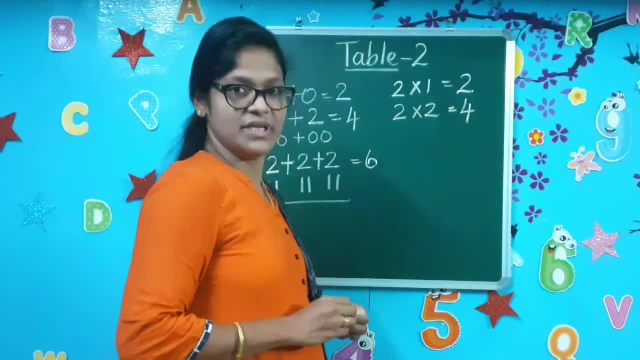 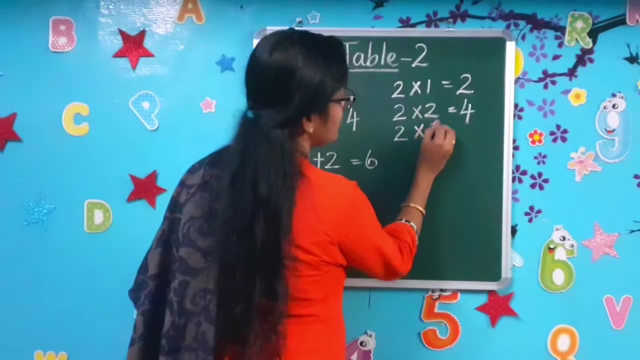 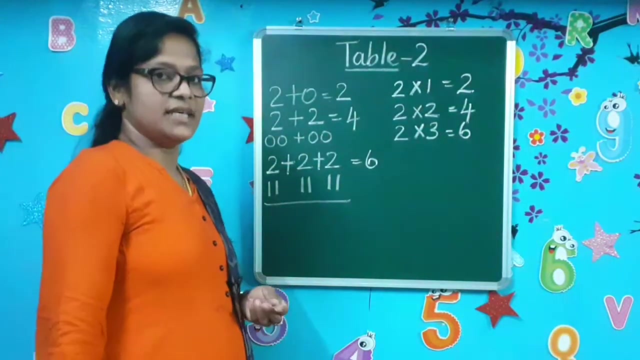 way, you have to learn the multiple table in the beginning. Okay, so I will just teach you 2,. how many 2s are here? 1,, 2,, 3, 3.. Okay, so 2- 3s are 6.. 2- 3s are 6.. Okay for the beginning. 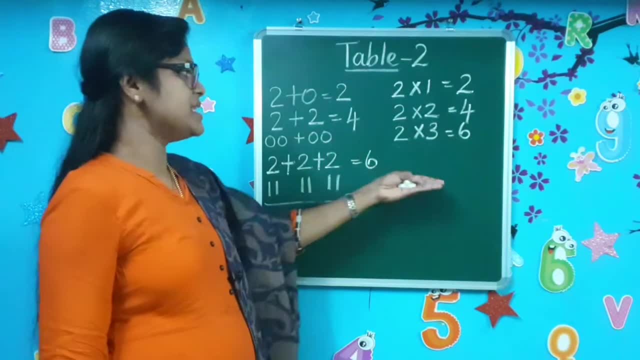 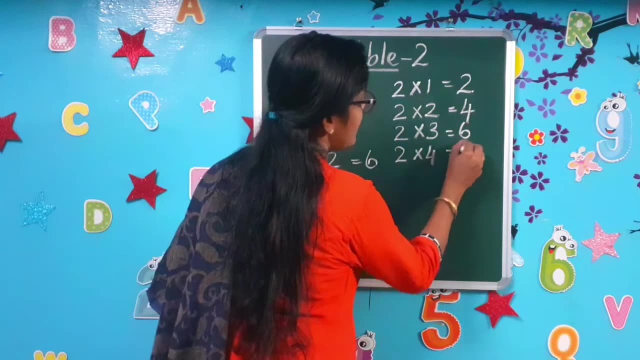 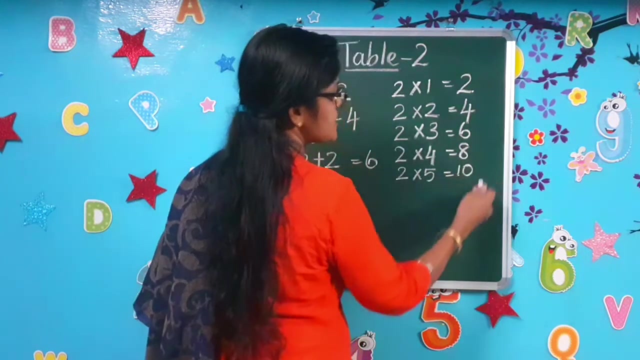 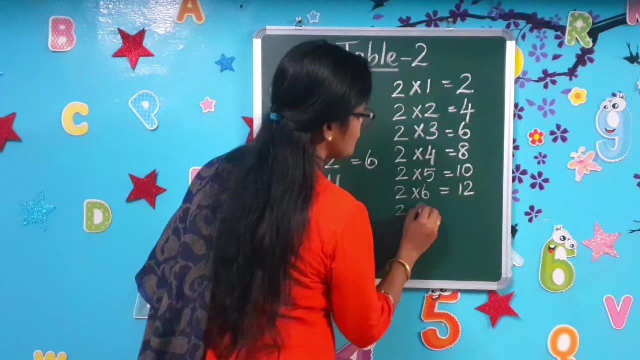 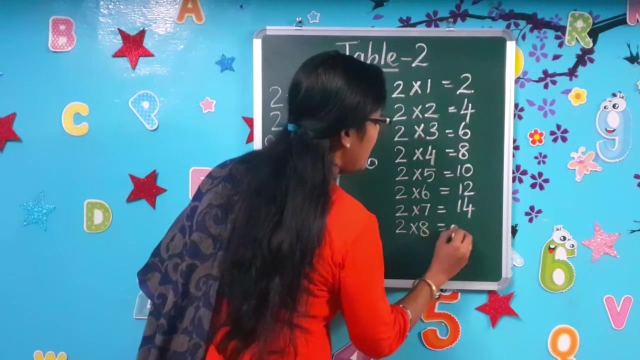 this is just for example. If you understand the concept, then it's easy for you. Okay, so next let's write: 2- 4s are 8.. 2- 5s are 10.. It isn't 2s counting, isn't it? 2- 6s are 12.. 2- 7s are 14.. 2 8s are 16.. 2- 9s. 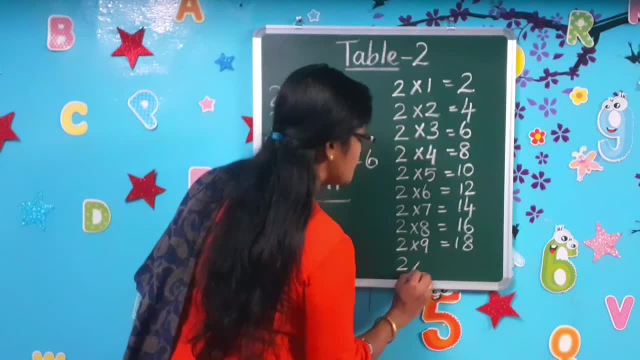 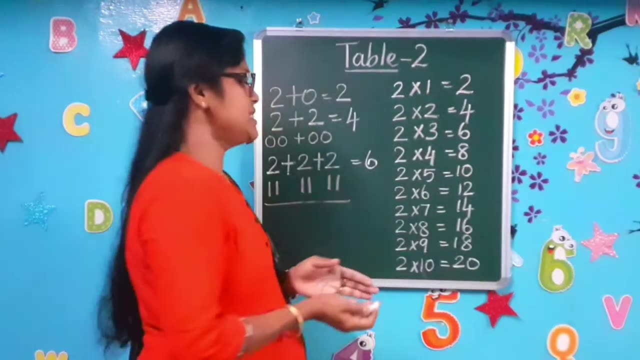 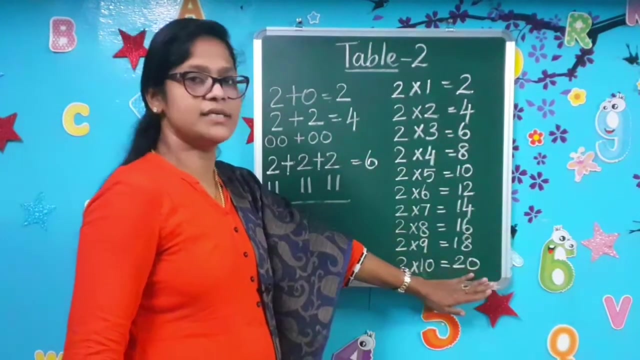 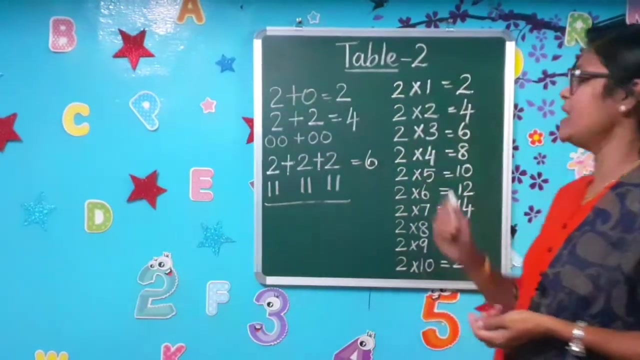 are 18.. 2, 2, 10s are 20.. Isn't it children? So as much as time you repeat them, you will identify how we are getting these answers. So that confusion, if it's there, then you would send repeated addition So you could just add the numbers. okay, Now see 2, 1s, 1s, you could add. 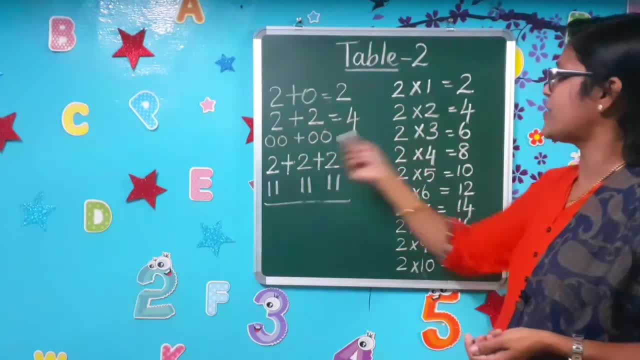 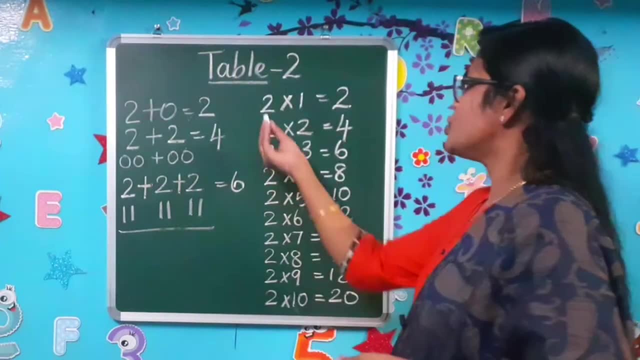 them: 2, 2s are So twice. you could write them: 2, 3s are Thrice. you could write them and count them and check whether the answer is correct. Okay, come on, let's repeat after ma'am: 2, table, 2, 1s are 2.. Say it after me: 2, 1s are 2.. 2, 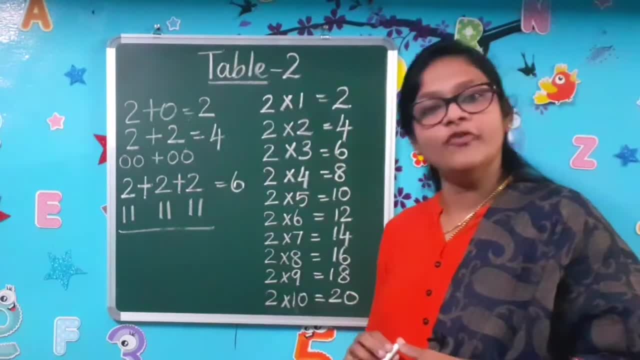 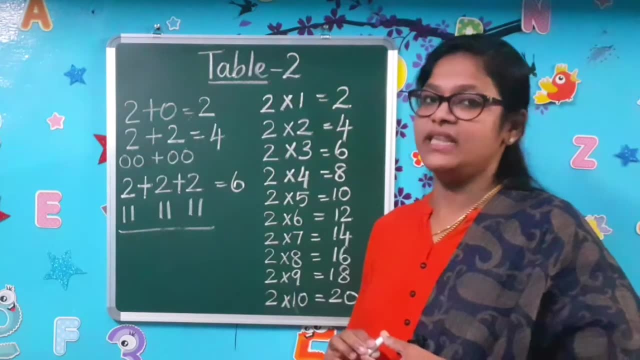 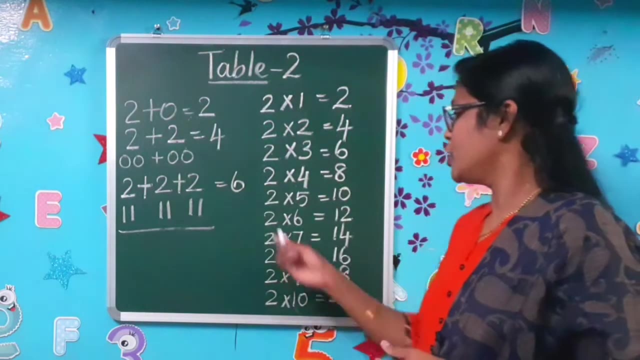 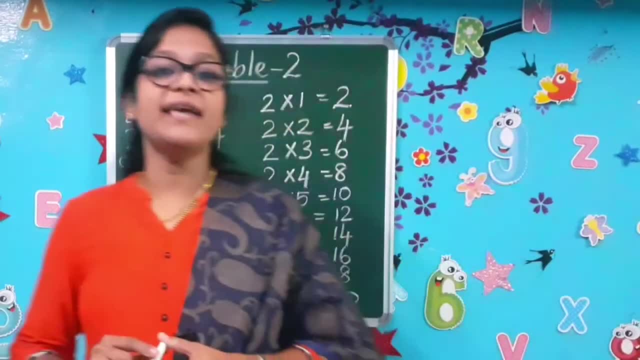 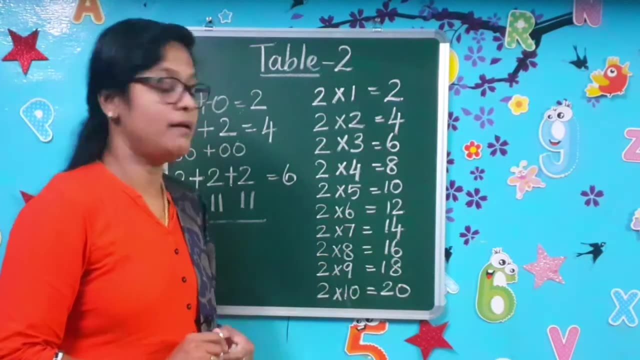 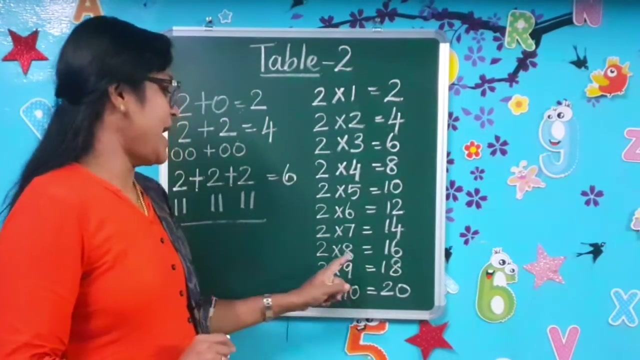 2- 5s are 10.. 2- 5s are 10.. 2- 6s are 12.. 2- 6s are 12.. 2- 7s are 14.. 2- 7s are 14.. 2- 8s. 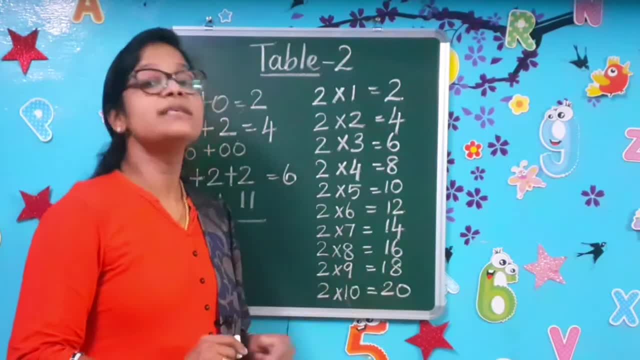 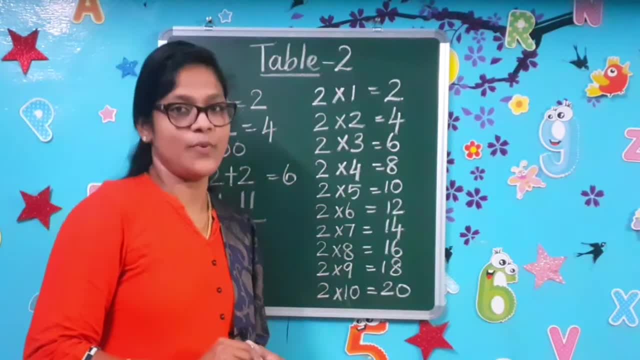 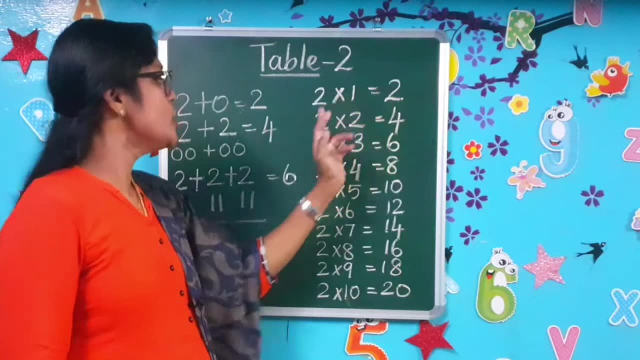 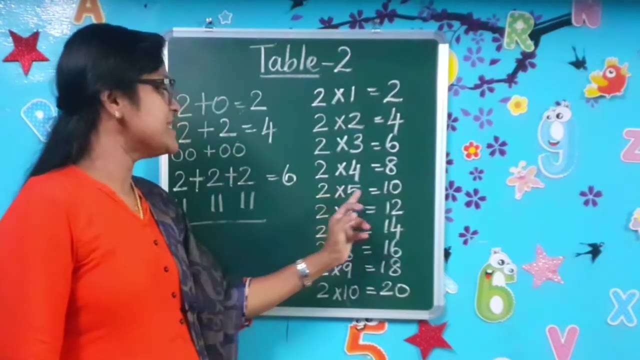 20.. 2 10s are 20.. 2 10s are 20.. Come on, let's sing it. 2 1s are 2.. Come on. 2 1s are 2.. 2 2s are 4.. 2 3s are 6.. 2 4s are 8.. 2 5s are 10.. 2 6s are 12.. 2 7s are 14.. 2 8s. 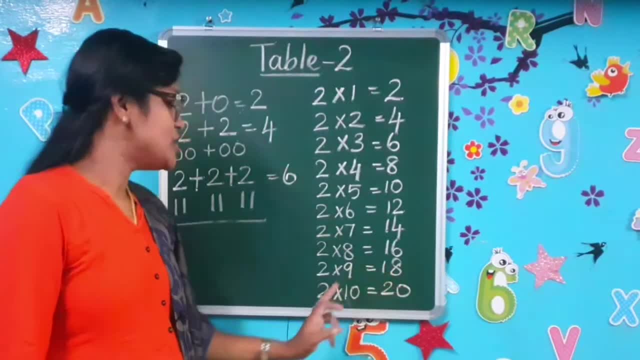 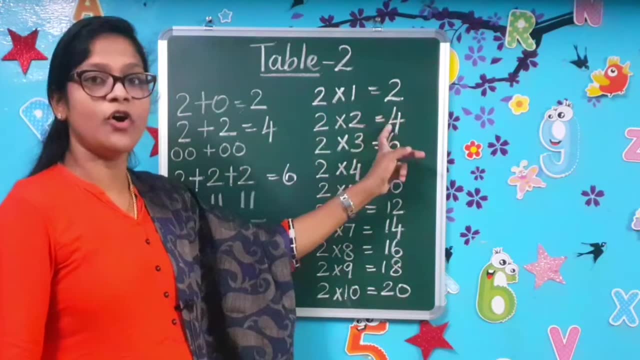 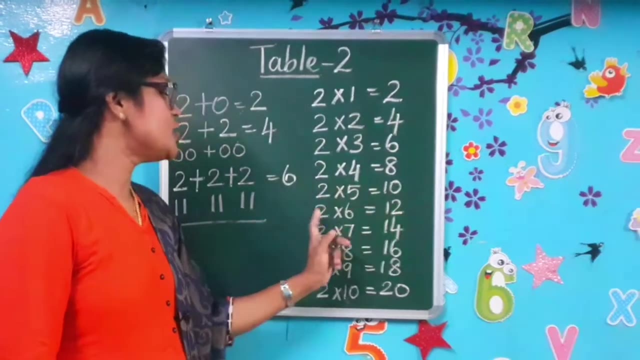 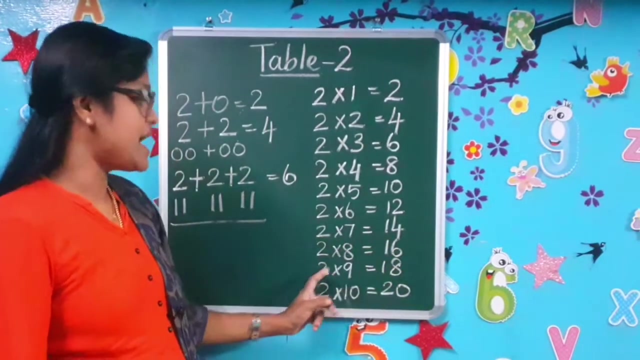 are 16.. 2 9s are 18.. 2 10s are 20.. Come on, let's sing it one more time: 2 10s are 20.. Come on, let's sing it once again: 2 1s are 2, 2 2s are 4, 2 3s are 6, 2 4s are 8, 2 5s are 10, 2 6s are 12, 2 7s are 14, 2 8s are 16,, 2 9s are 18, 2 10s are 20.. 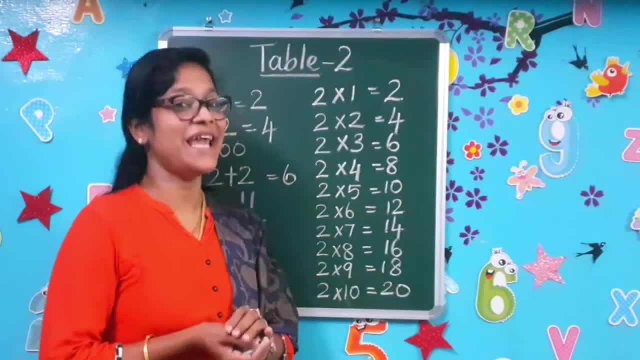 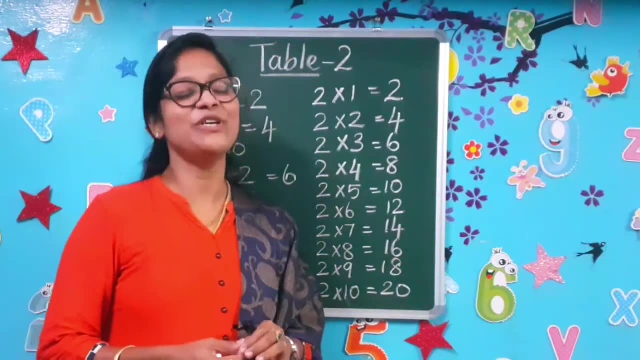 Okay, my dear kids, I hope you will sing and learn the multiple table easily. Okay, keep practicing and learning the multiple table. See you all soon in the next class with the next table 3.. Bye, bye, kids, bye, bye, take care, bye, bye.